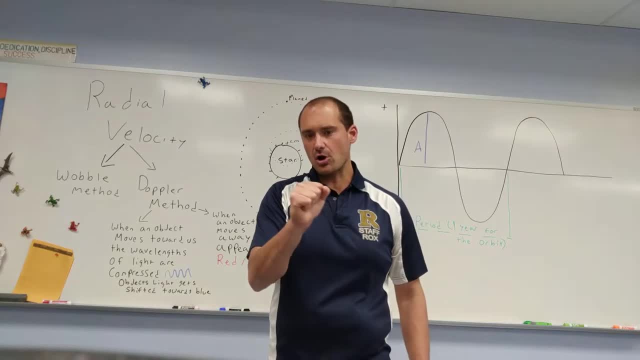 of starlight caused by the sun or star orbiting its common center of mass. When that star is moving towards us, it's blue-shifted. When it's moving away from us, it's red-shifted. 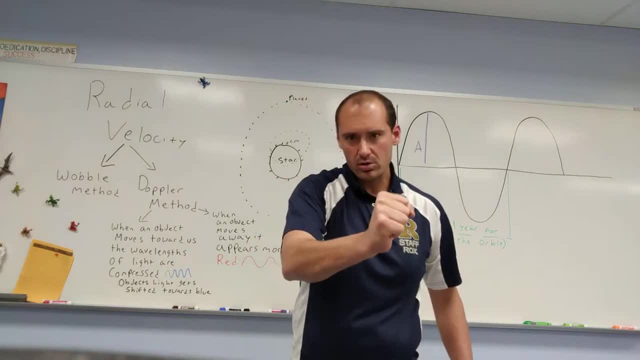 And the greater the Doppler effect, the greater the wobble, the more you see this blue-shifted effect. 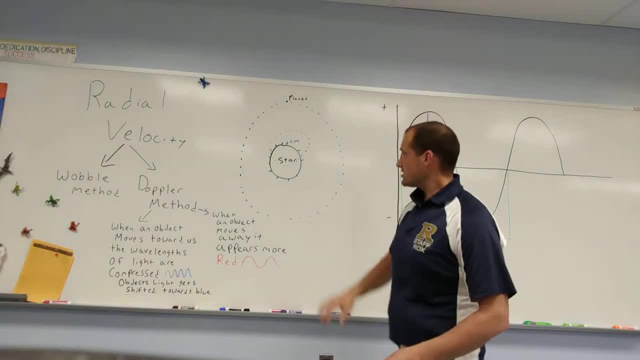 So what I've shown you here in a little bit of a drawing is just, we've got a star and we've got a planet, and this star is orbiting around the common center of mass, and of course the planet, as well, is orbiting around the common center of mass. When the planet is 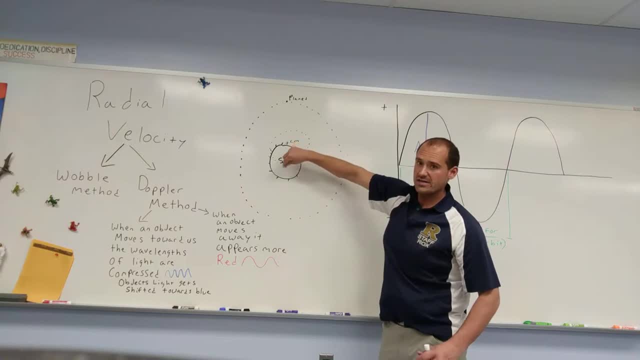 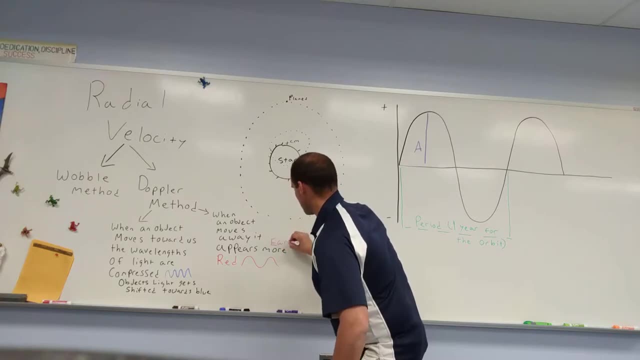 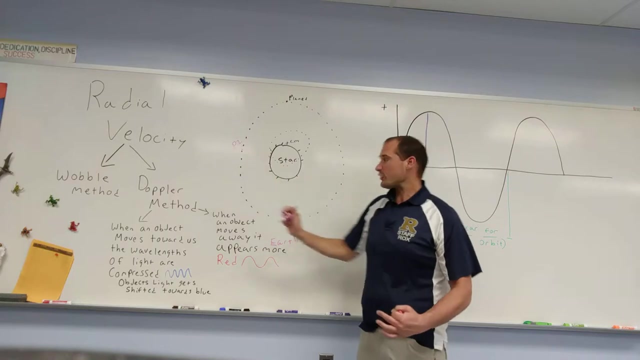 at this part of its orbit, you'll notice that the star is actually closest to us. So if you could imagine, like, Earth being in this general direction, you'll notice that the planet is at the same point, in the same direction, however, as it's moving away from us. biliares. In some 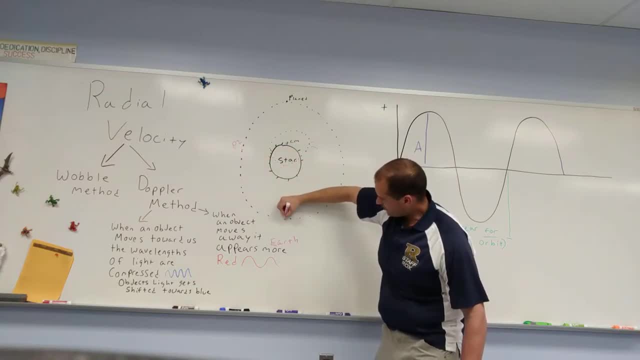 places you'd think that the star rounds around. Just understand tha with the tail of your eye and the pointy-anks, it's whole on the other side of the planet. It's not even moving at us anymore because it's kind of moving side to side. So we don't detect a Doppler shift at that point. I'll show you what that looks like on the graphs. 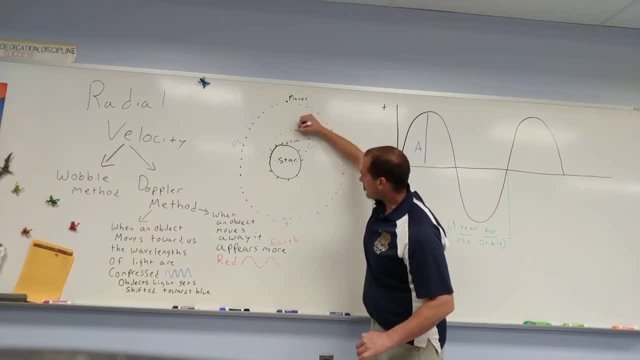 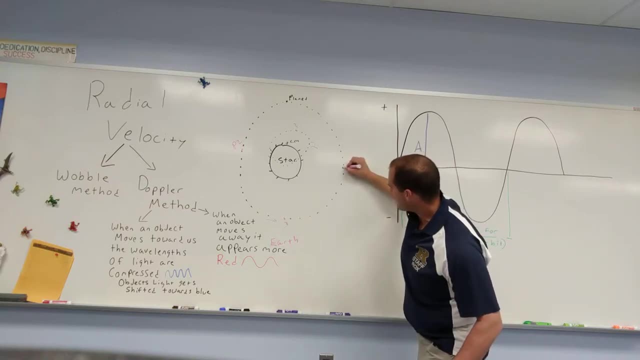 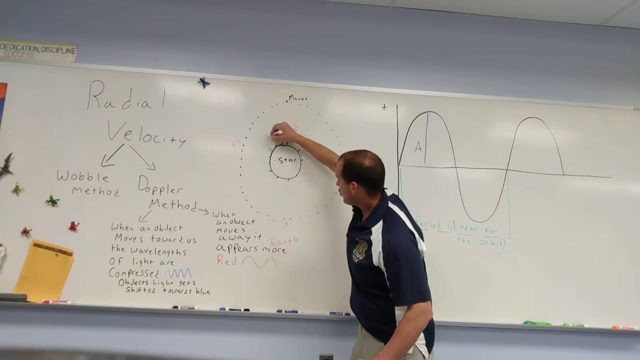 Our star has now moved as far away from us as it could have. Now that planet's going to continue swinging around, moving away from Earth. And our star is now going to start moving towards Earth. And we're going to start seeing a blue shift because that light is moving towards us. The light is being compressed. And we can show this in the graphs. 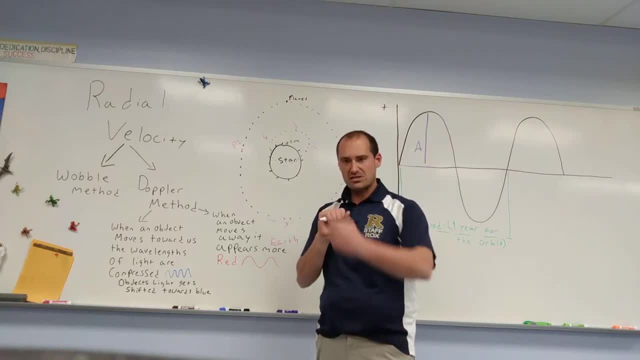 So this type of motion is called reflexive motion. As the planet moves towards you, the star moves away from you. And as that planet moves away from you, the star moves towards you. And you're going to see that in the graph. 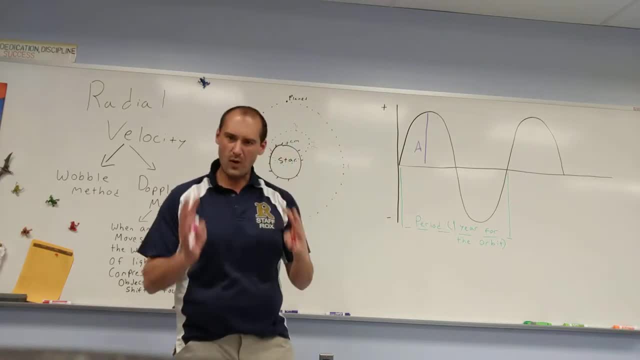 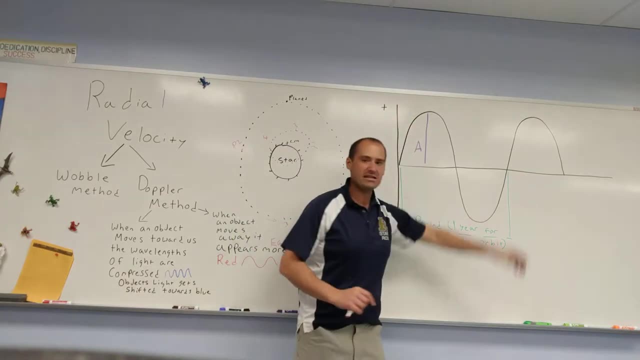 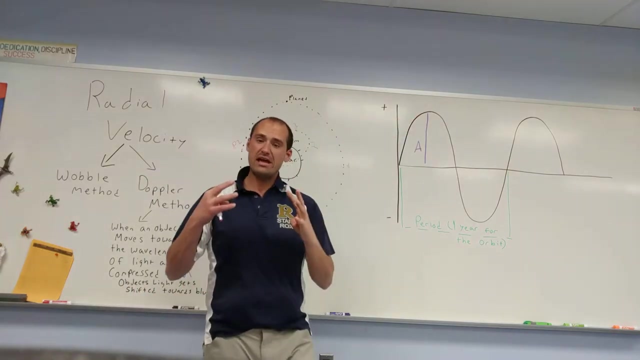 Now the graph I have here is a graph of the wavelengths of light. And you'll notice it has a positive signature and it has a negative signature. Some words that you're going to want to know for this. The height is called amplitude. 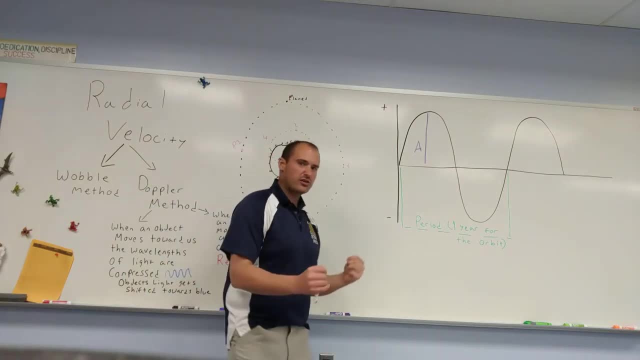 That's basically how blue shifted or how red shifted. Is it? 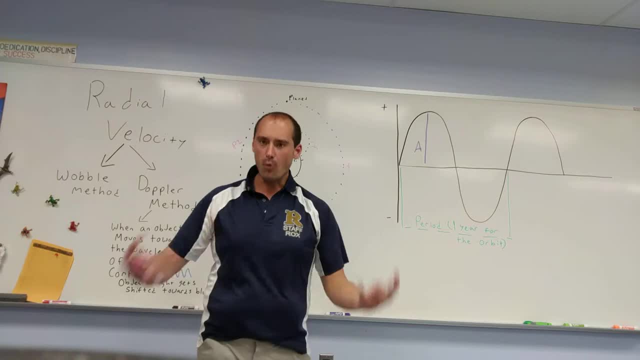 The greater the blue shift, the greater the red shift, the more the wobble. That means that planet has to be tugging pretty hard on its star to wobble more. 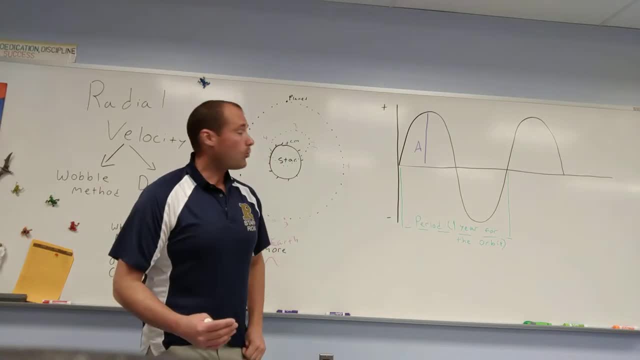 And the period. Basically it's the time when the planet goes around the star once. Or the star completes a full orbit. I've picked from here to here where it returns back to that original position as my period. But you could have done from here to here as your period. 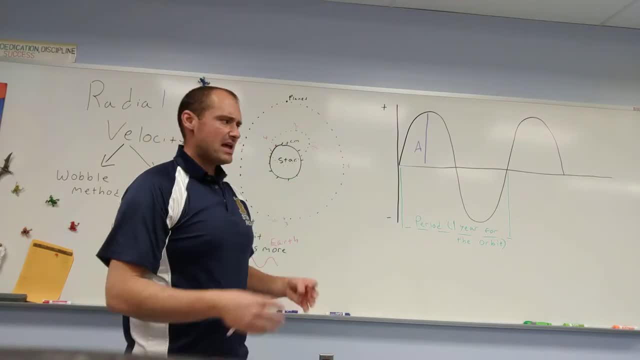 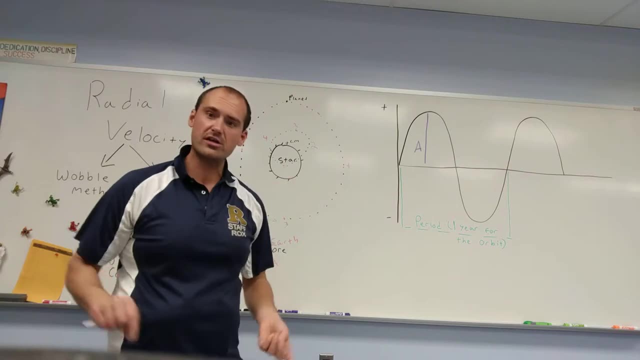 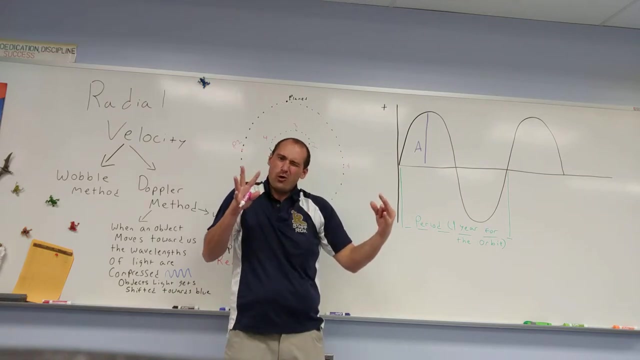 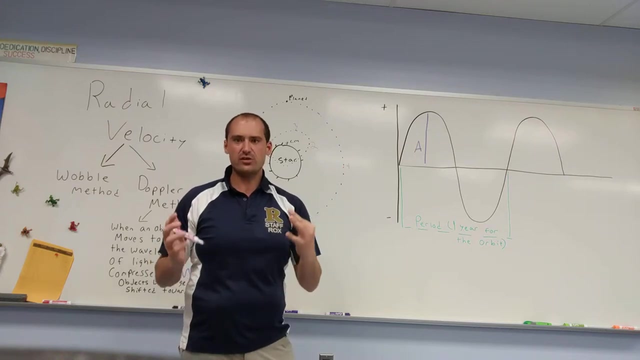 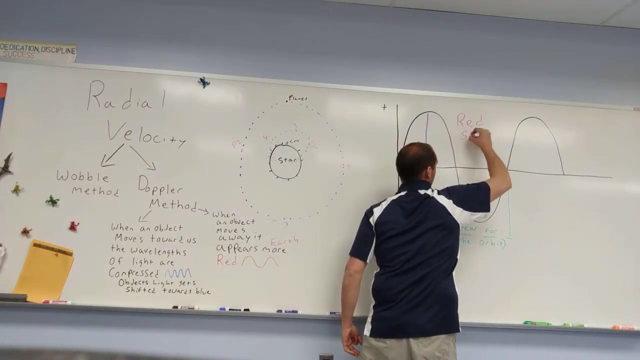 Again, it's just getting back to that original starting position. And on the simulation that we do in class, I believe it actually tells you the period. I think it actually even gives you the number. You can calculate it if you really want to go that way. You'll notice up here this positive signature means the light waves have been stretched out. And when they're stretched out, is that red shifted or blue shifted? If you said red shifted, you're right. So the top of the graph, this area of the graph, is when the star is red shifted. 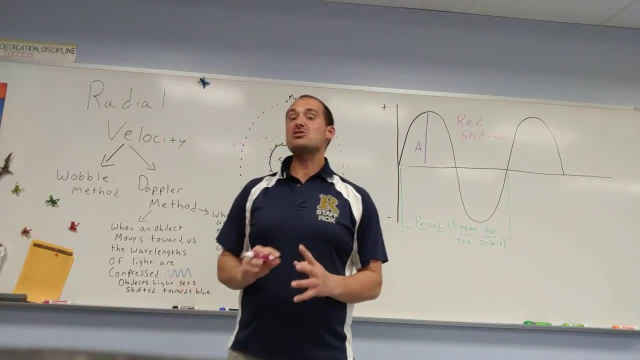 And when the star is red shifted, that means the star is moving away from us. It's moving away from us. 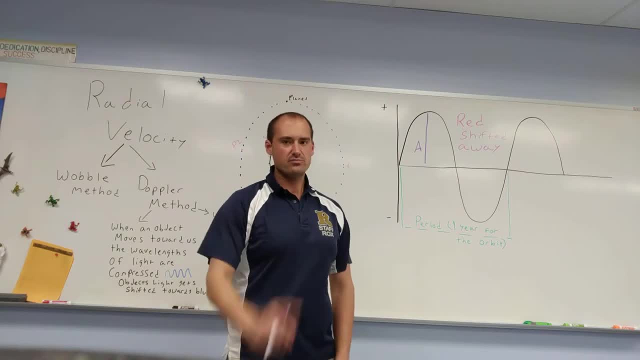 Now you may ask yourself, Mr. Killifin, what is the planet doing? Hashtag reflex of motion. 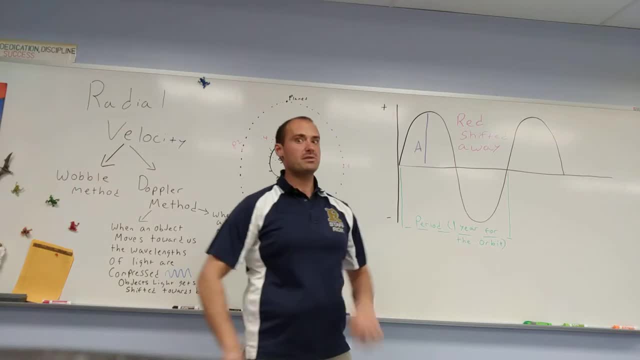 If the star is moving away from us. The planet must be moving at us at this point. 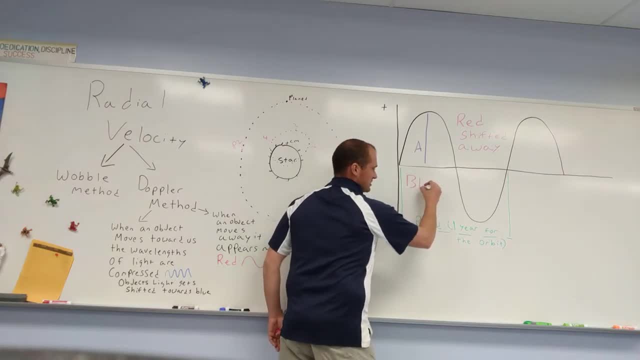 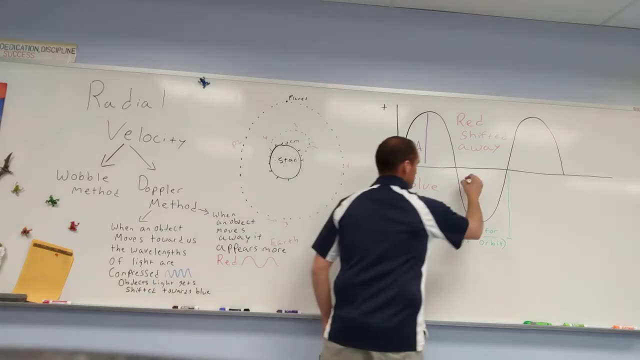 Down here, you probably guessed it, the wavelengths are compressed and you're getting, you're observing a blue shift and that means the star is moving towards us and the planet is moving away from us. 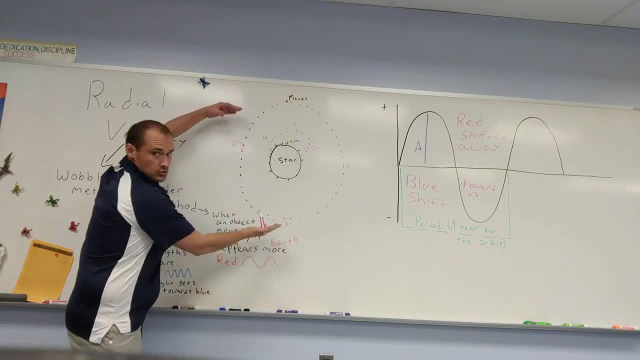 If we really wanted to graph this and take a look at how it relates to the little chart that I've done here, think about it. 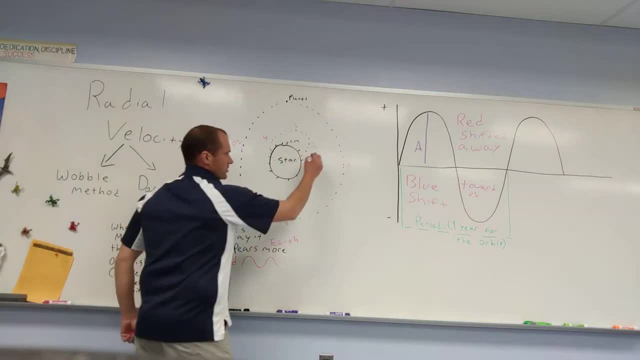 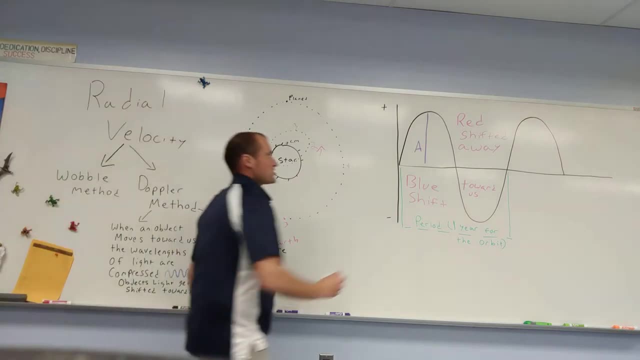 At time two for the star, this is when the star is moving the strongest away from us, the fastest away from us. 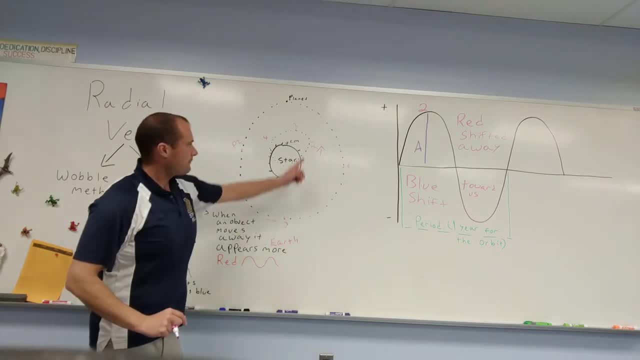 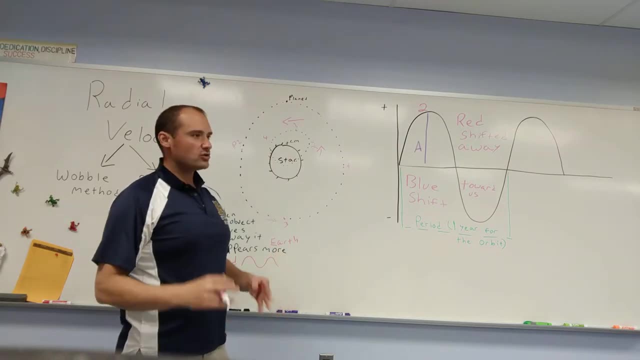 This would be time two. By the time it gets over here, it's not moving away from us, it's not moving towards us, so we don't see a Doppler shift. 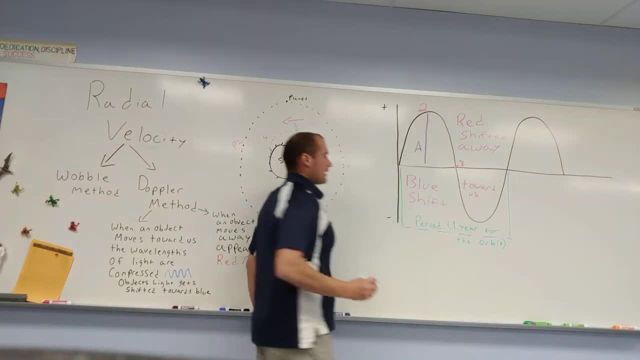 So time three could best be represented by this. Okay. 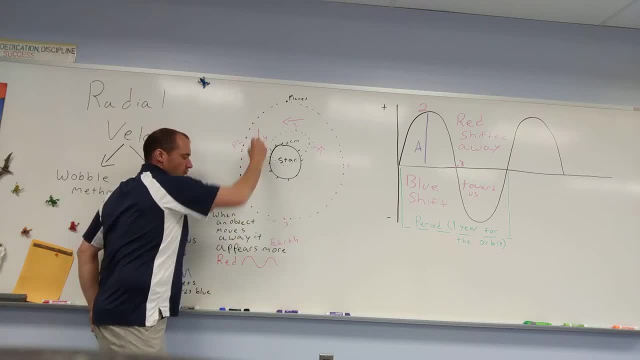 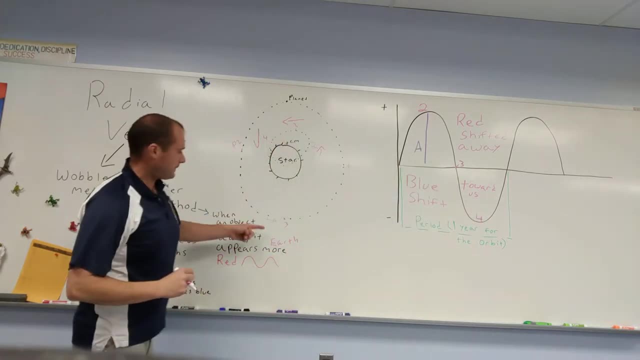 By time four, the star again is moving at earth. So we see a blue shift and by time three, it's moving kind of to the side of earth. So we're not seeing a shift at all. 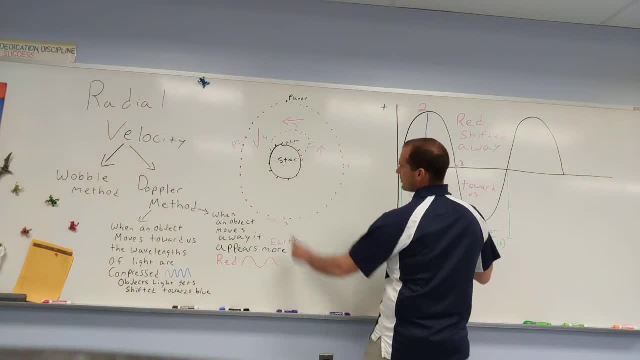 You could say that time, what did I do here? 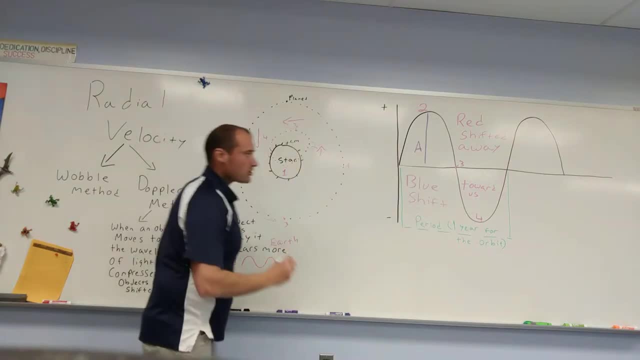 Oh, excuse me. I had the original starting position here. Time one being right, right there. Time one being right, right there. Time two being right, right there. Time three being right, right there. Time four being right, right there. Time five being right, right there. 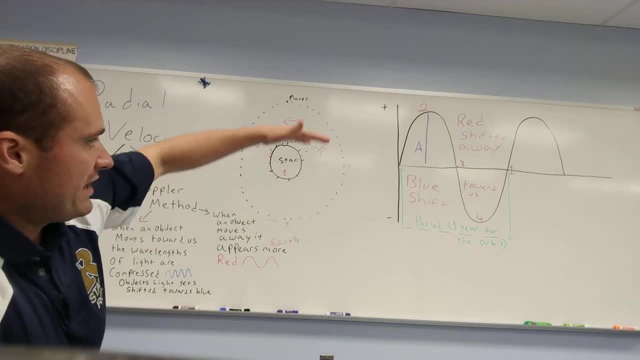 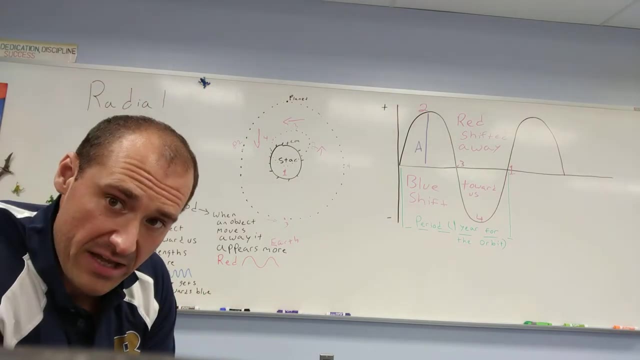 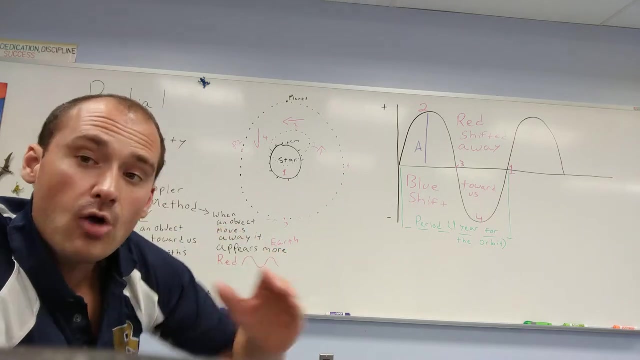 What you'll probably notice is that the higher the amplitude, the larger the mass. The closer the planet is to the star, the tighter that period is, the smaller that period is. 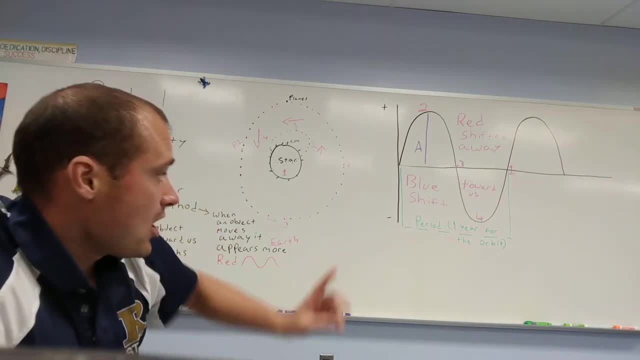 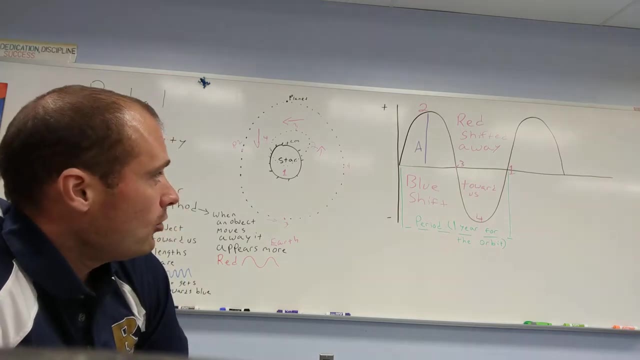 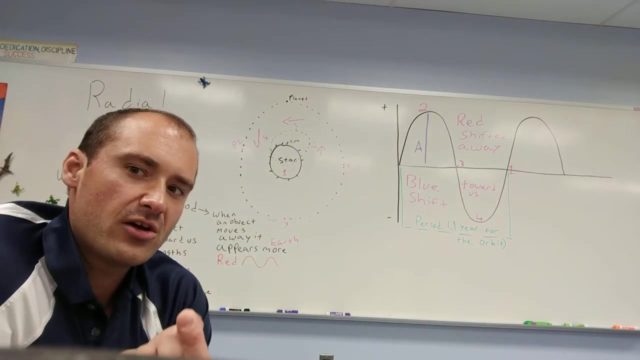 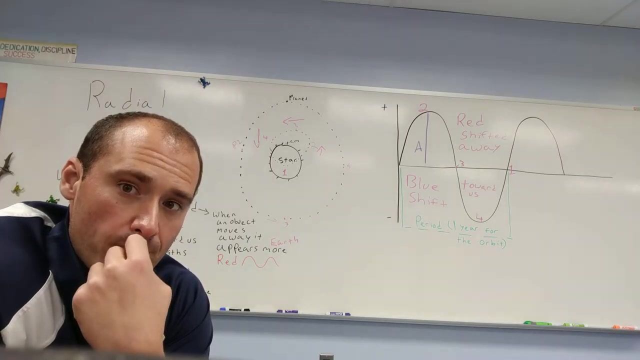 Remember, when we started doing Kepler's laws, the period of the planet is related to the distance from the planet. So if we know the period, we can tell the distance and by looking at the amplitude, you can tell the mass of the planet because that planet is causing its star to gravitationally wobble. 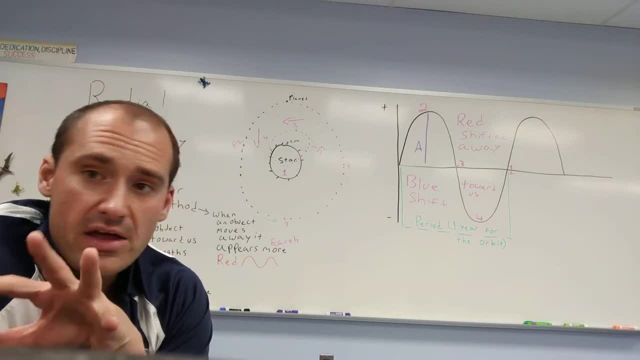 A couple of problems with this method. 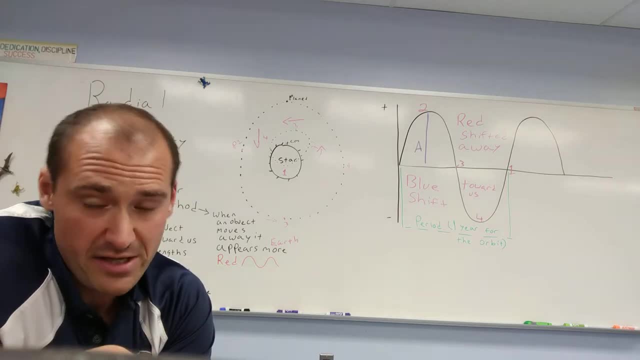 This method is biased towards large planets. Why? Well, because large planets are going to be easier to detect. If you're a large planet, you're going to cause that star to wobble. 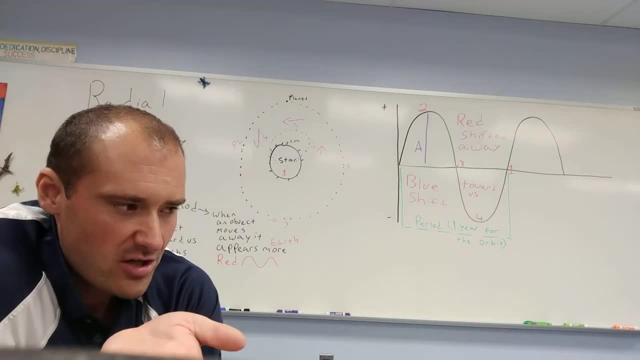 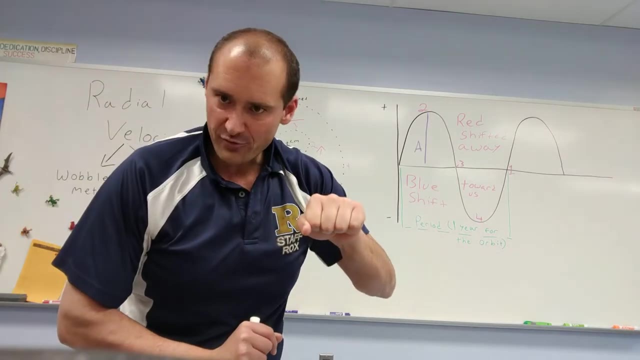 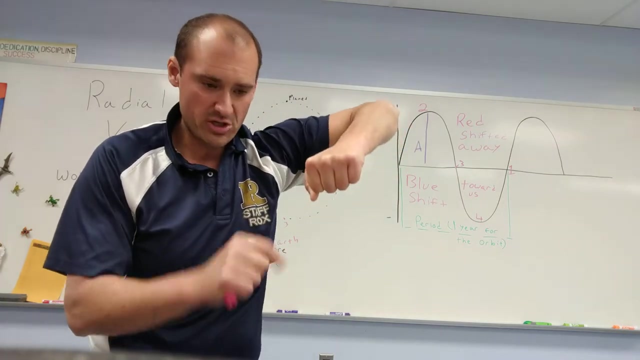 It also doesn't work for systems that are not oriented directly at us or away from us. If it's tilted, some of that wobbling motion is coming at us and some of that wobbling motion is just kind of going in the down direction. So we detect a lower mass than that planet really is. So I may tell you a planet is four masses of Jupiter. That's the minimum mass that planet could be. That's the minimum size for that planet. That's the minimum mass that planet could be.